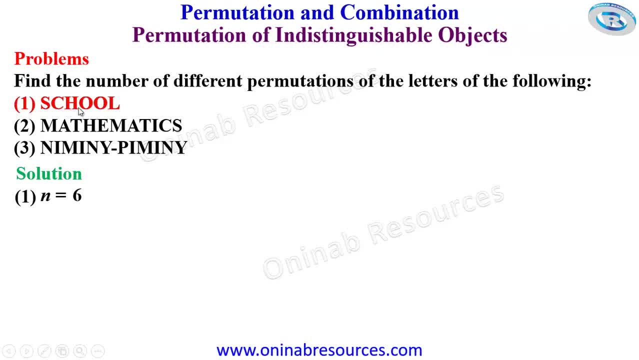 15 math 16, 17 math, 18, 19, math, 19, 20, math, 21, 22, math, 22, 23, math, 24, 25, math, 26, 27, math, 27, 28, math, 29, 30, math, 30, 28, math 31. 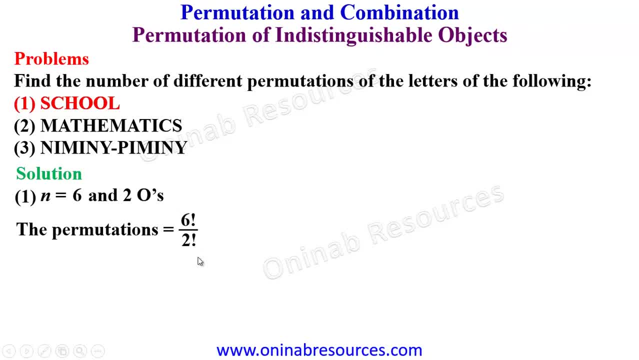 33, math 32, 33, math 37, 38, math 39, 40, math 41, 38, math 42, 38, math 42, 39, math 42, 39, math 43, 40, math 44. We are then having 360 permutations. 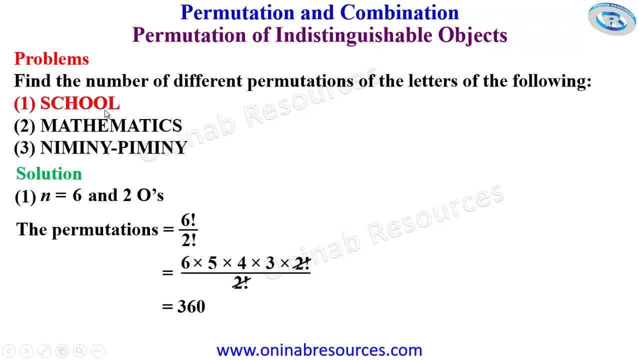 There are 360 permutations of the letters of the word school. Then we go to problem two, mathematics. So we count the number of letters: 1, 2,, 3,, 4,, 5,, 6,, 7,, 8,, 9,, 10,, 11.. 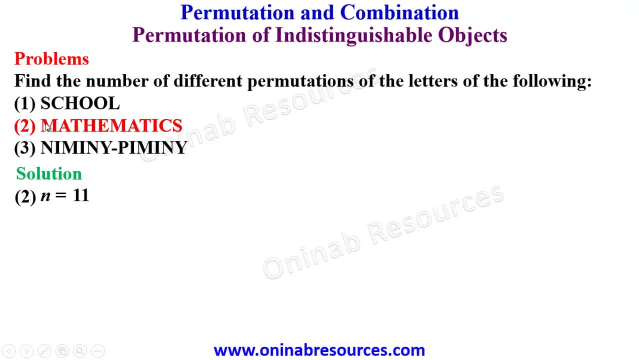 So n is equal to 11.. Then, how many m's do we have? We have two m's. How many a's? We have a, two a's. How many t's? We have two t's. We have one h, one e, one c, one i and one s. 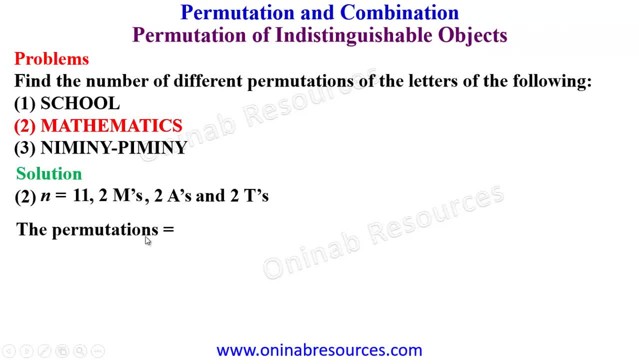 So the number of permutations now will be 11 factorial over 2 factorial, 2 factorial, 2 factorial. If you, If you input this in our calculator, we have our solution as 4,989,600 permutations of the letters of the words mathematics. 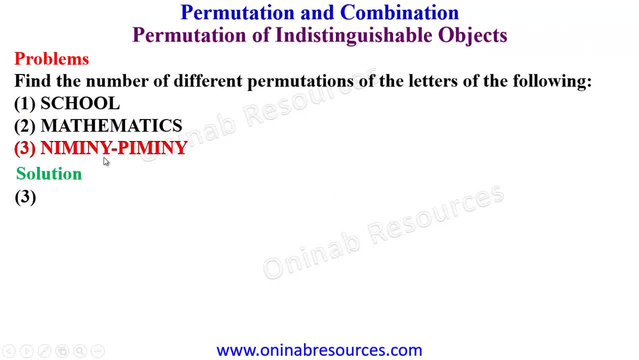 So we go to problem three, that is, nimini-pimini. We count 1,, 2,, 3,, 4,, 5,, 6,, 7,, 8,, 9,, 10,, 11, 12.. 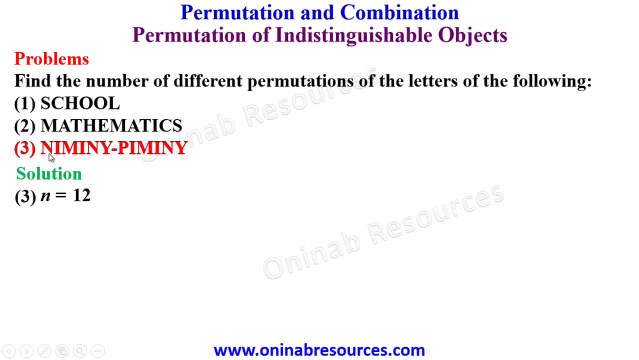 So our n is equal to 12.. Then we now see we have 3 n's, So we have 3 n's, 4 i's, we have 2 m's and we have 2 y's and only 1 p and 2 y's.